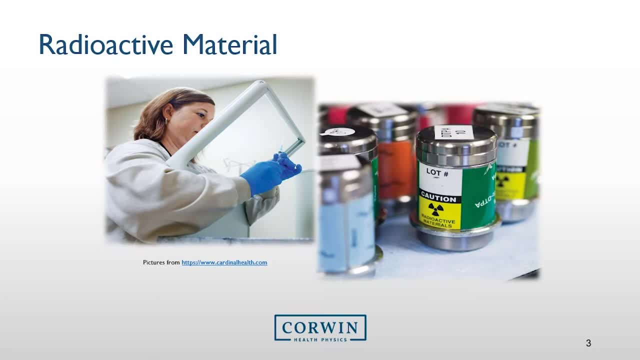 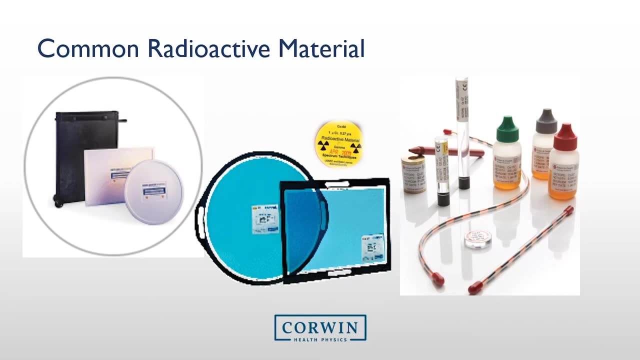 may contain radioactive material while performing their duties. Here are some common radioactive material sources. All these sources should be stored properly in a designated area, usually the hot lab. All these sources should also have a radiation symbol on them letting you know it is radioactive. 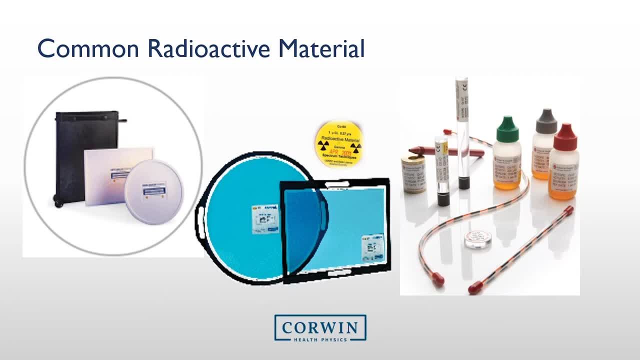 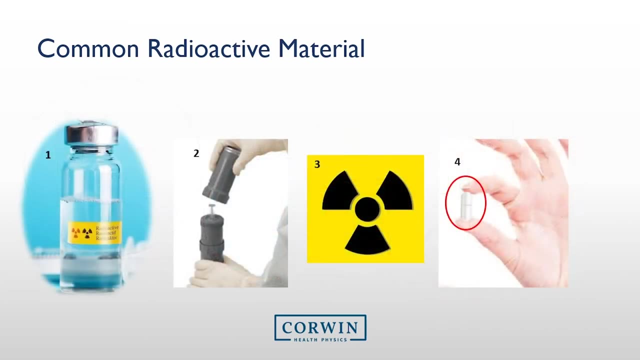 But, as a reminder, housekeeping and other ancillary staff should not come into contact with these sources pictured here, as their duties do not take them into the hot lab, and the sources are all handled and stored by the nuclear medicine technologist. Here are some more examples of radioactive material used in the nuclear medicine department. 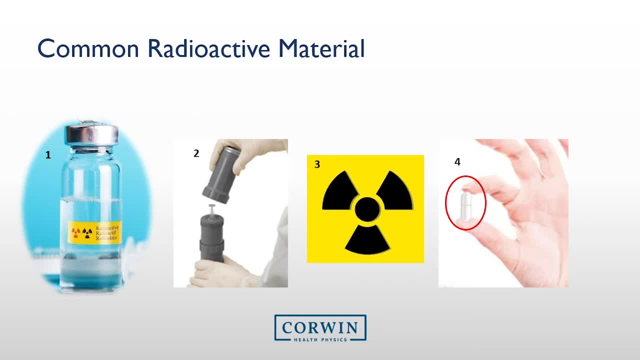 Here are some more examples of radioactive material used in the nuclear medicine department. Some sites will order radioactive material in a 10 cc vial, shown here in Figure 1.. Most sites will order unit doses in a syringe depicted in Figure 2.. 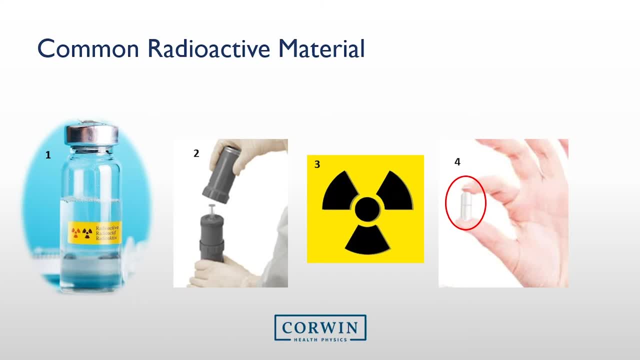 All radioactive material should have a radioactive sign that resembles Figure 3.. However, some radioactive material comes in the form of capsules and some radioactive signs are described as capsules- capsules as seen in Figure 4.. They arrive on site in a radioactive labeled container. 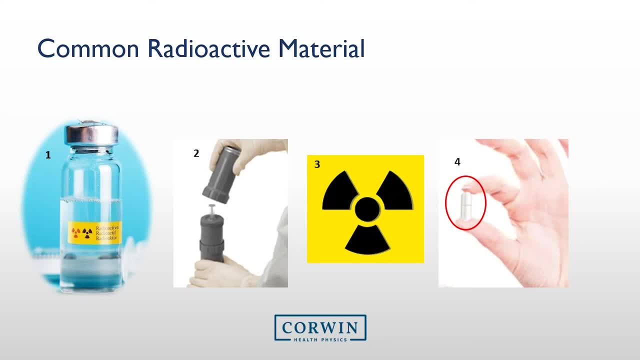 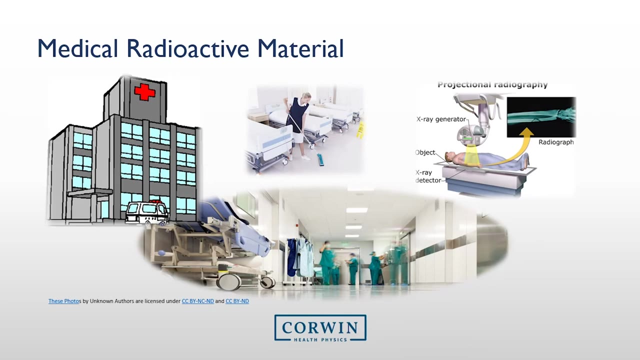 but once outside the container they can look like any other capsule. If capsules are found around the nuclear medicine department, as a precaution, treat it as radioactive material. Radioactive material is used only in the nuclear medicine department and very rarely in angiospecials. 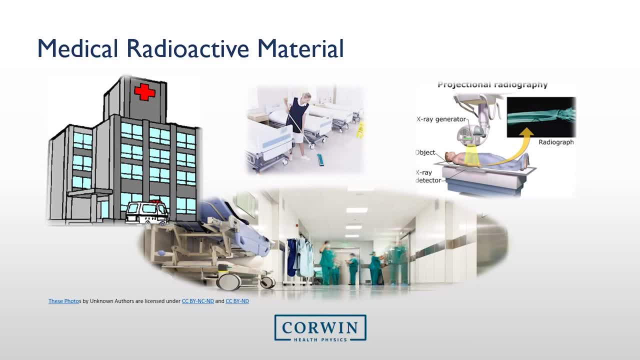 labs for therapy purposes. No radioactive material should be in any other location at your facility. Note that x-ray systems do not contain radioactive material and only cause x-rays when they are turned on and the x-ray control button is pushed. There are no radiation hazards near an x-ray system that is turned off. 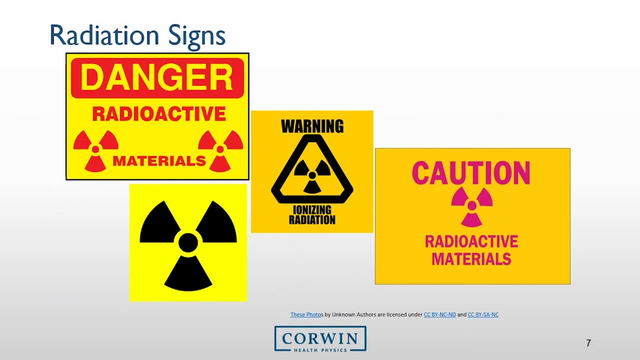 Here are some radioactive signs you may see in the department. Sometimes these signs produce fear and anxiety, but rest assured that in all the areas where your duties take you, the nuclear medicine technologist performs daily surveys and spill checks to ensure the department is safe from contamination. Their job and goal are to keep